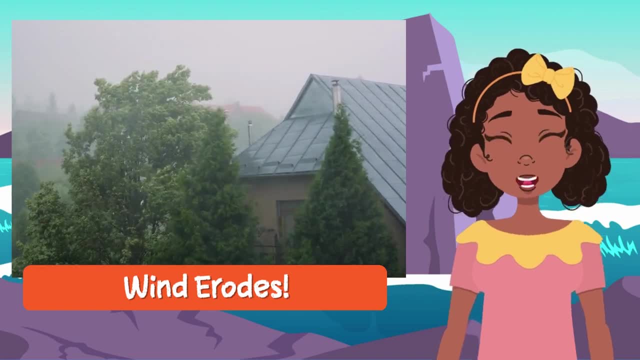 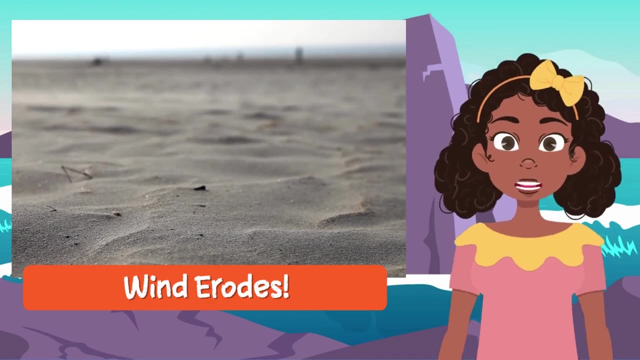 or it can be strong and powerful like a storm. What is wind? Wind is a force that moves things around. It can be strong and powerful like a storm. When the wind blows, it can pick up and move tiny bits of rock and soil. In fact, it can. 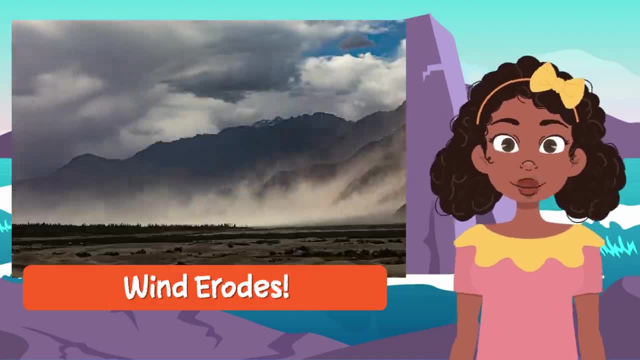 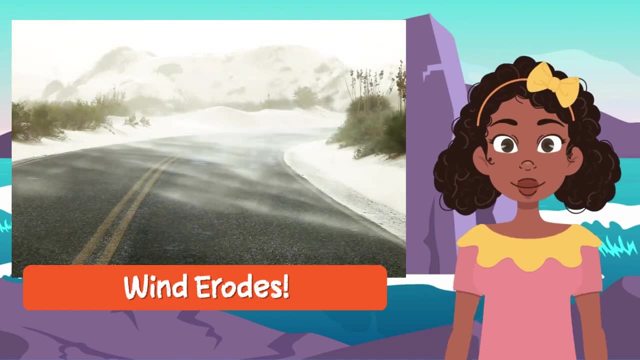 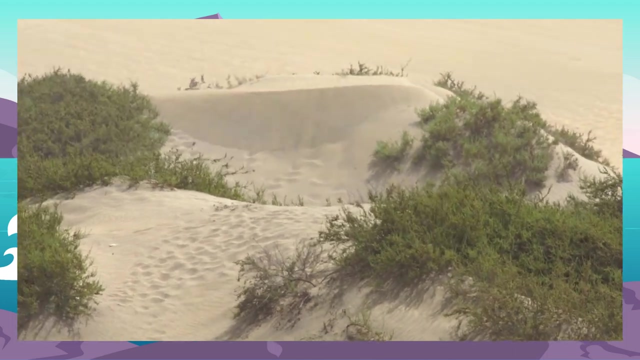 carry these pieces really far away before finally dropping them. That's erosion: moving materials from one place to another. The tiny bits of sand and rock that the wind carries can be really powerful. They can blow against landforms or they can blow against rocks. 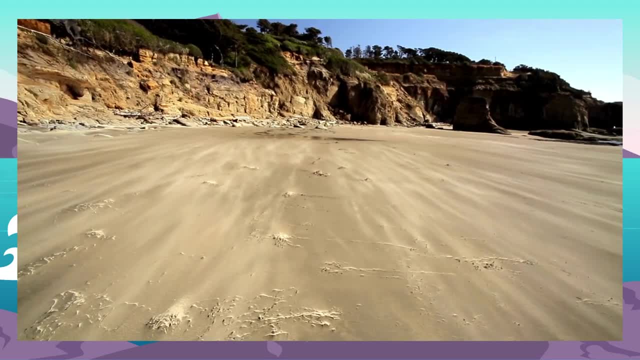 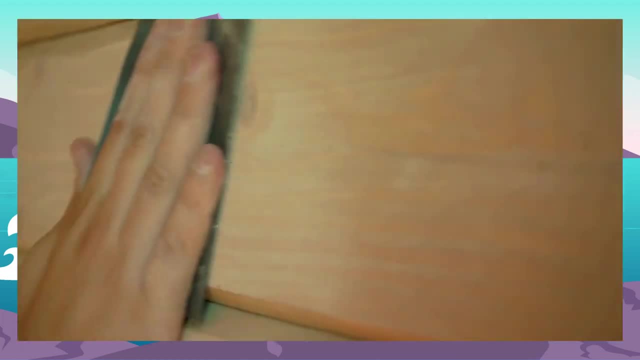 When the winds blow, they carry these pieces of sand and rock. They then drop them off on the ground and wear them away. This process is called wind weathering. It's like taking a piece of sandpaper, rubbing it against something and wearing it down Over time. the wind can weather rocks until 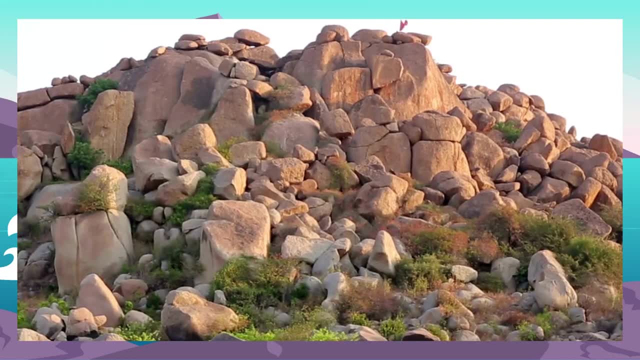 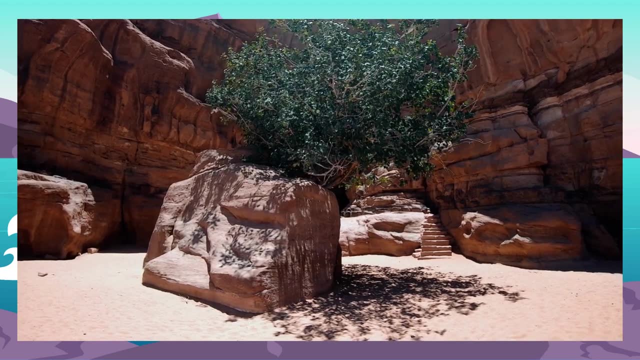 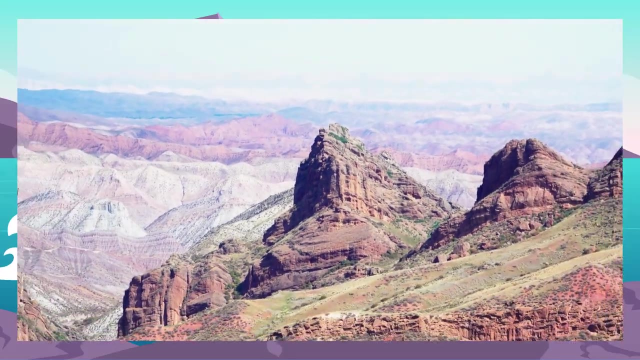 they become smooth and flat. Wind weathering tends to happen close to the ground because it's not powerful enough to lift the soil and rocks it is carrying very high. When the wind carries the particles, They hit the bottoms of larger rocks, slowly carving out unique shapes which can be really fascinating to look at. 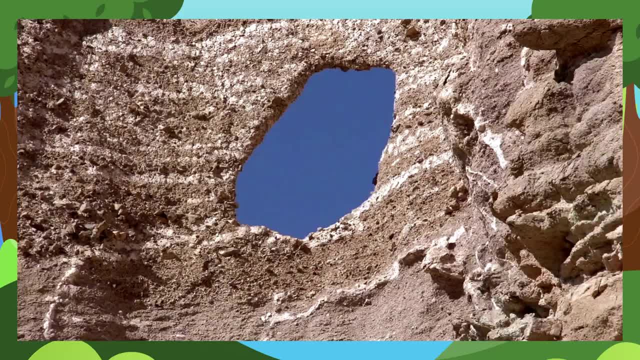 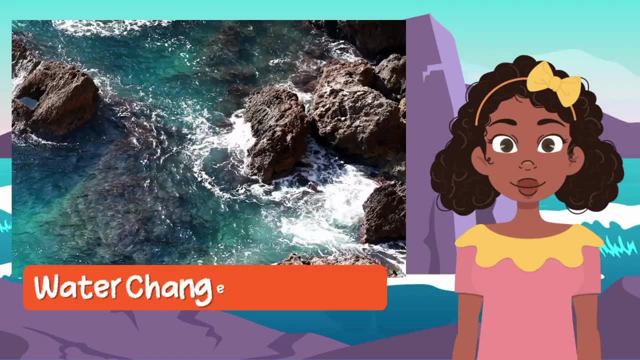 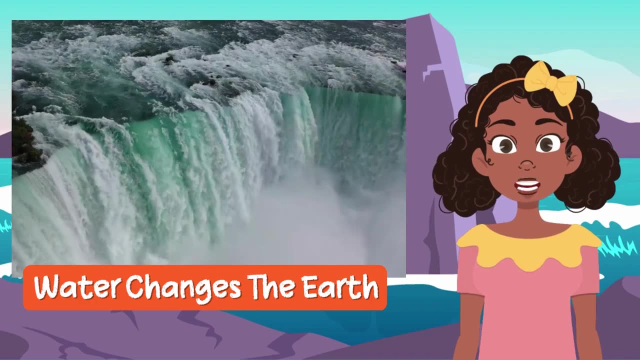 Weathered rocks come in all shapes and sizes. Some of them have holes in the middle of them, while others look like mushrooms. Water changes the earth Just like the wind. water can cause weathering and erosion. Water covers almost three-quarters of our wonderful earth. 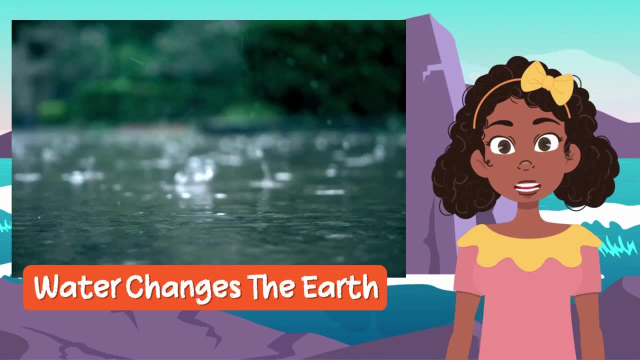 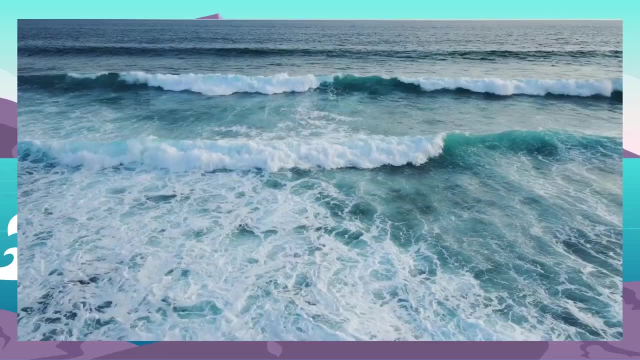 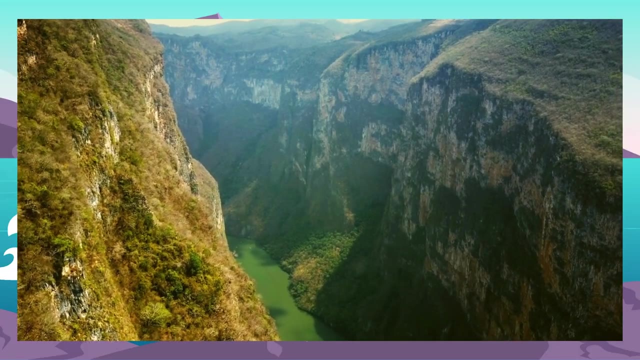 It falls to the ground as rain and snow and flows through rivers and streams. It also swirls around in the ocean. As it moves, it helps to shape and change the surface of our planet. Water can help to form canyons and hills, shape mountains and can even make new land by depositing sediment. 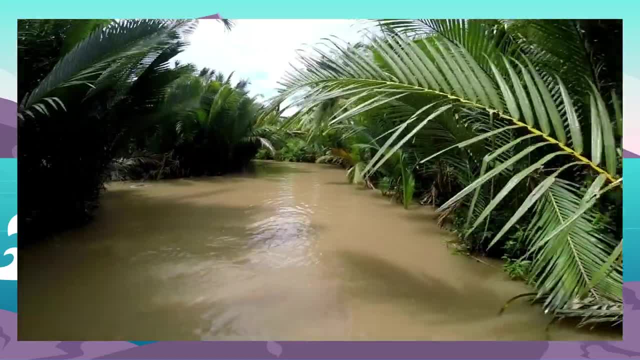 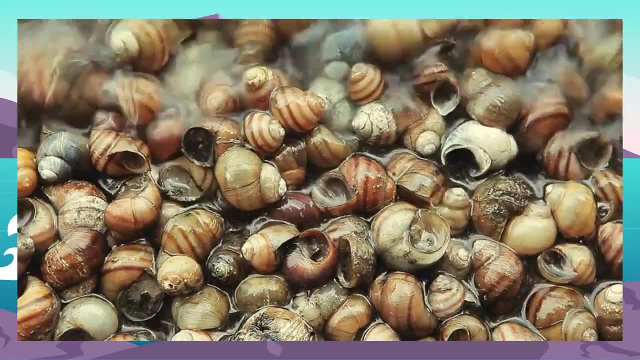 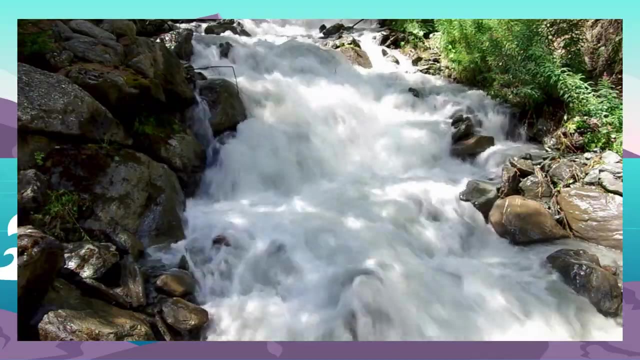 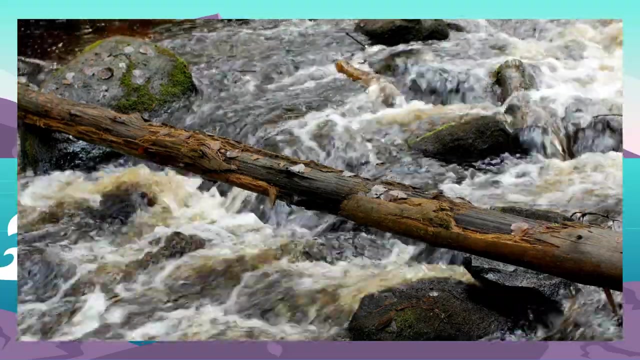 Sediment can be made up of all sorts of things that the water carries, like sand, dirt, rocks and even shells. The faster the water moves, the more the water can carve away at the rocks and land around it. Streams and rivers are bodies of moving water that can wear away even the sturdiest of rocks over many years.